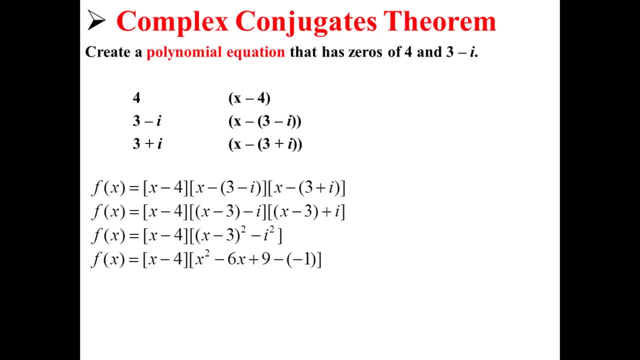 Now we factor this out to get x minus 4 times x, squared minus x, squared x squared minus 6x plus 9 minus negative 1.. We simplify further to get x minus 4 times x, squared minus 6x plus 10.. 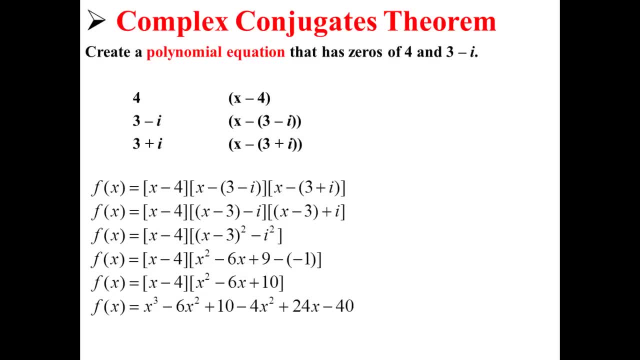 And now we follow that out to get x to the third minus 6x squared plus 10 minus 4x squared, plus 24x minus 40.. Finally, we simplify that fully to get x to the third minus 10x squared plus 24x minus 6x squared. 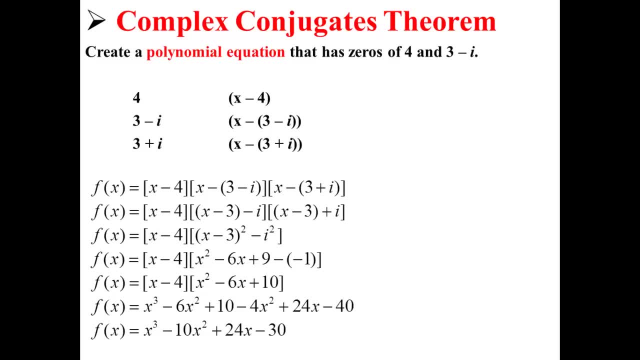 And now we've created a polynomial equation that has zeros of 4, 3 minus i and 3 plus i. 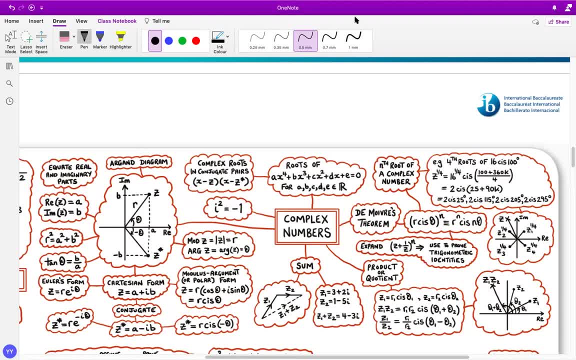 Hi, hope you're doing well. Well, in this sub-fragment I'm going to cover up the basic concepts of complex number for AAHL syllabus- AAHL- part of your TP course. Now what is the main breakdown for the course? the other content that we have here. 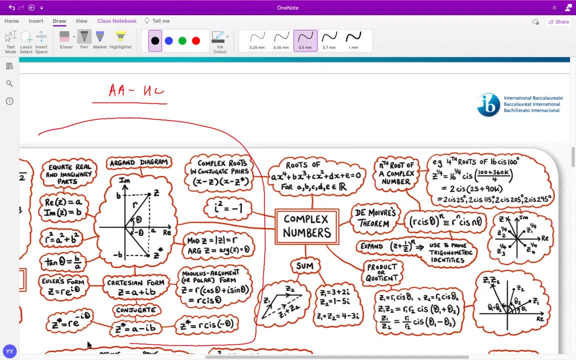 So the first part is that links up the basic part of the complex number. I would say that this is this is going to be in my first video. This is the second part that I'm going to cover up, That's your polynomials and all, And I'm going to take the third part, which is where the most of the 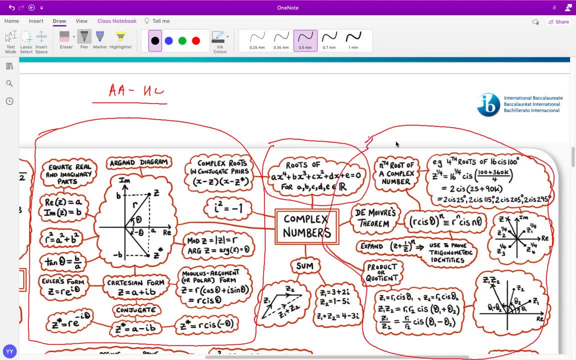 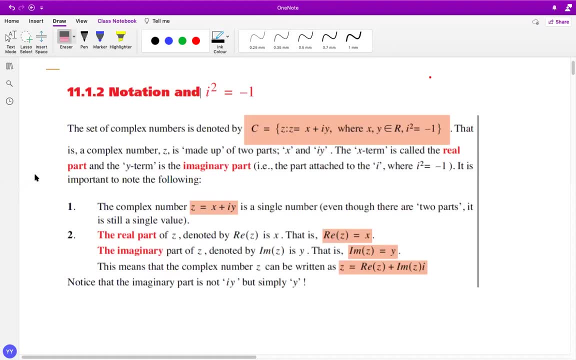 section B type questions are asked in IB are going to be on De Moivre's theorem. So I'm going to take make four videos on these topics where you can watch the concepts and some of the IB problems on the same. So let's begin off with the basic introduction about the complex number system.